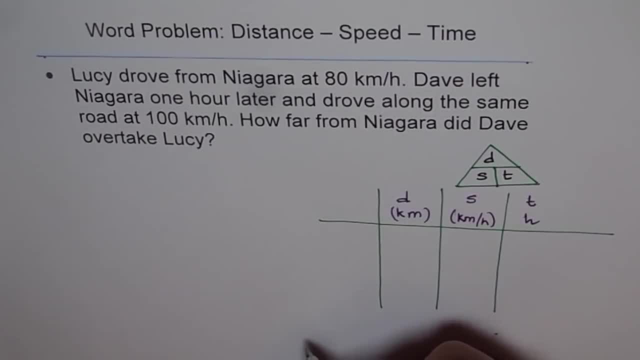 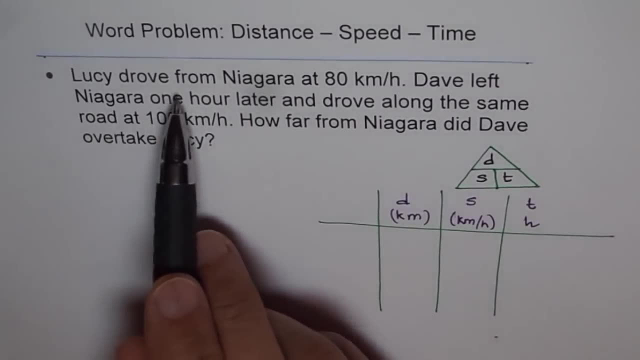 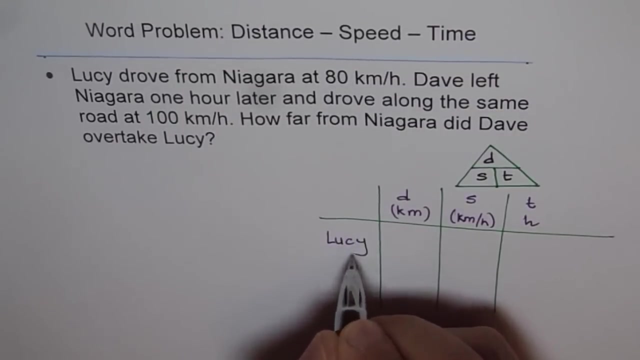 And time, which is in hours. right, And now let's read the problem to translate all these things in tabular form. It says Lucy drove from Niagara at 80 kilometers per hour. So Lucy, speed given is 80 kilometers per hour, correct, 80 kilometers per hour. 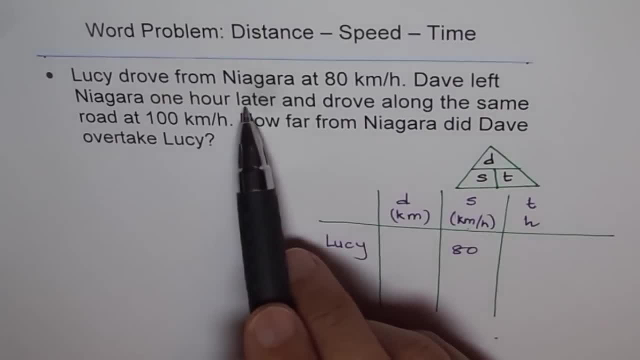 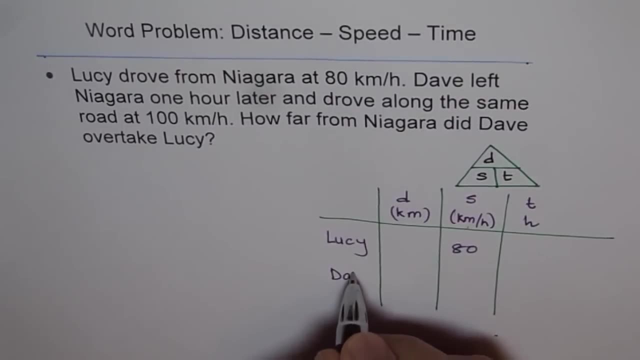 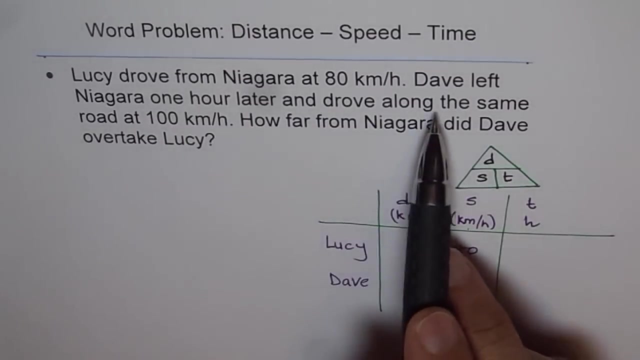 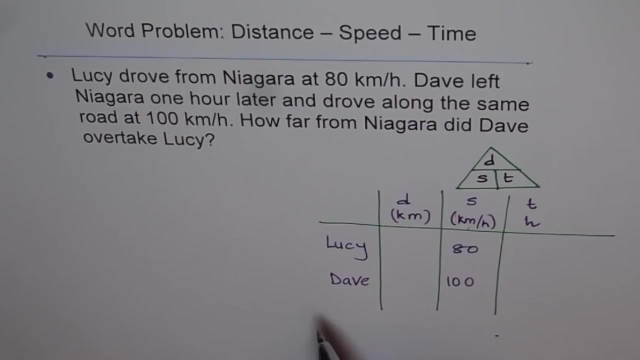 Then Dave left Niagara one hour later and drove along the same road at 100 kilometers per hour. So let's say Dave drove at 100 kilometers per hour. Now it says left one hour later. What does that mean? That means we need to define our variables, like time. 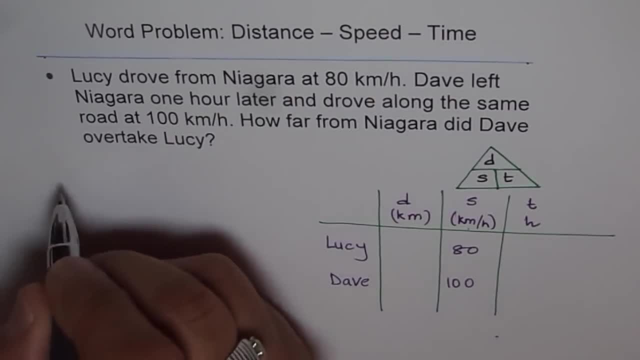 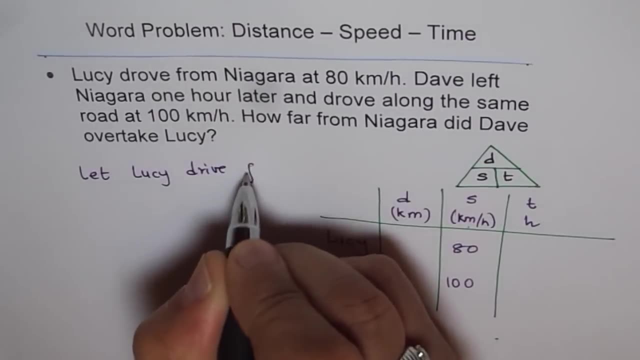 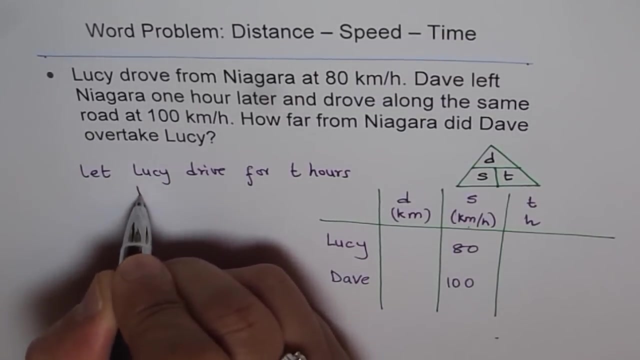 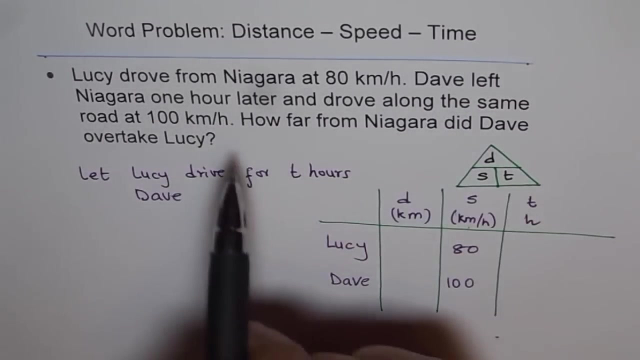 We don't know how much time did Lucy take. So say, let Lucy drive for t hours, Then Dave will drive. for how long? Dave left Niagara one hour later. What does that mean? What does that mean One hour later? So will it be t plus one or t minus one? 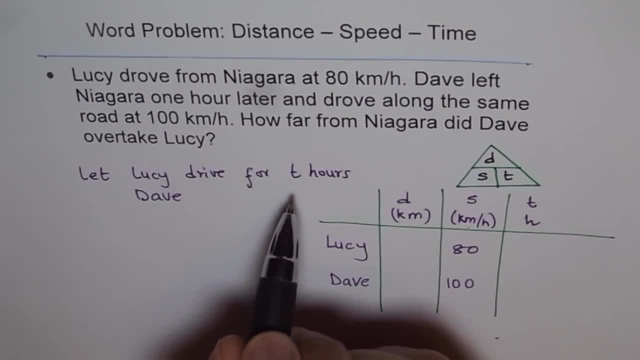 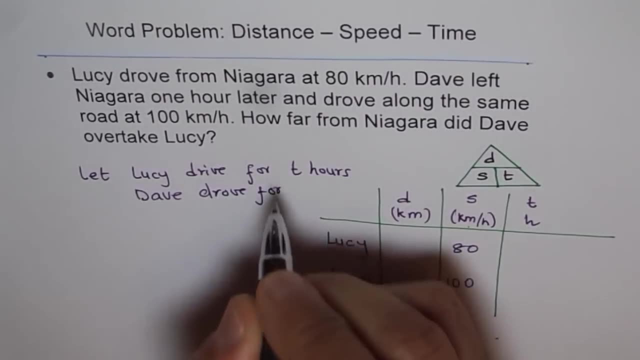 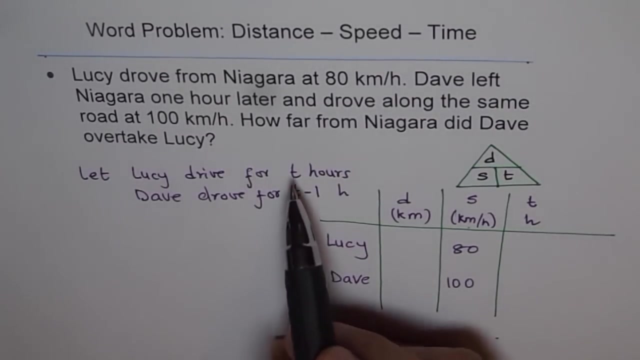 One hour later means he took one hour less. He drove one hour lesser, correct? So Dave drove for t minus one hour. Do you understand that aspect? Or you could use two variables. You can say t one for Lucy, t two for Dave, and then we can relate them later, right? 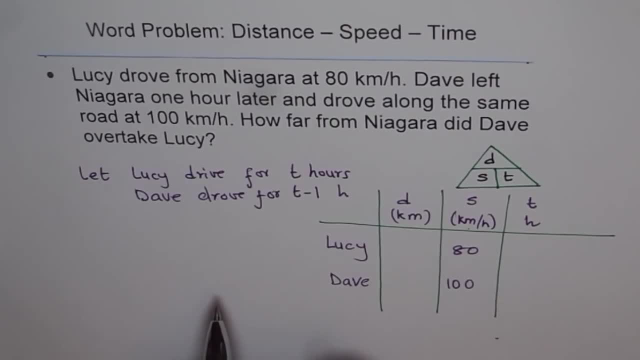 So that could be done using two variables- One hour later, One hour later variables- but at present I think that is good enough. we say Dave left Niagara one hour later, so whatever, if they are driving for the so. so that is how their times are related, so they will be. 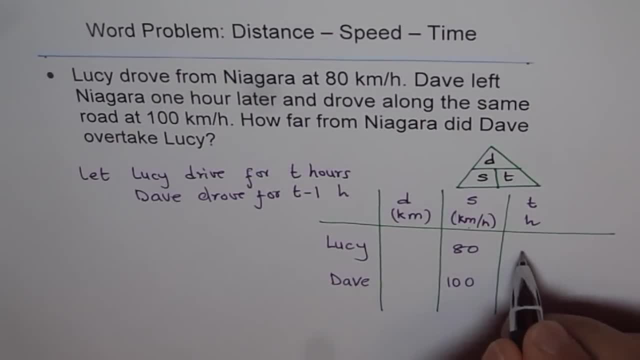 one hour less than Lucy. so say, Lucy takes t hours and they will take t minus one hour. right, let's read the problem further. how far from Niagara did Dave overtake Lucy? so at the time when Dave overtakes Lucy, they must have covered the same distance from Niagara, because they started from. 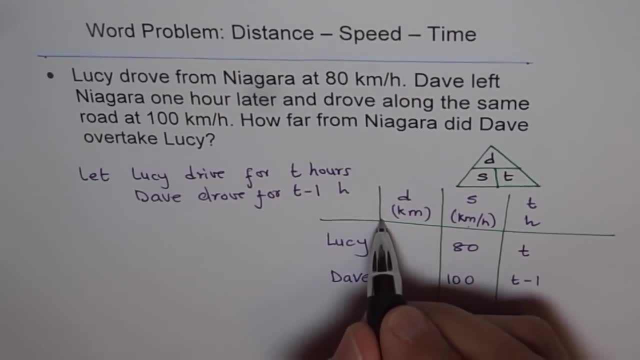 the same place, right, good. so let's say: this is our starting point and and let's say here: Dave overtakes distance, traveled is same. do you see that same distance? so we will say that Dave overtakes Lucy and Lucy overtakes Lucy. and let's say here: Dave overtakes Lucy. 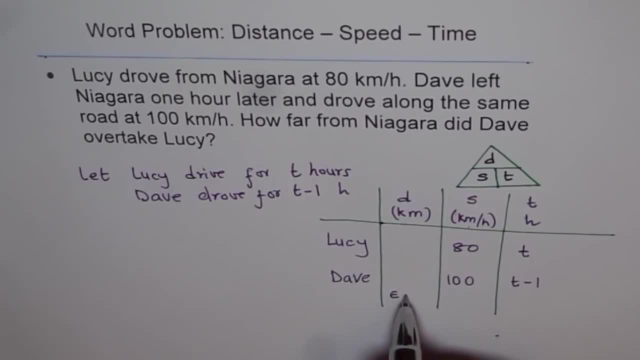 say: well, at that time these distances are equal for both of them. So that will make our equation correct. Now, what is distance? Distance is speed into time. So Lucy will cover how much distance? 80 times t. So the distance covered by Lucy will be 80 t. The distance covered by Dave will be: 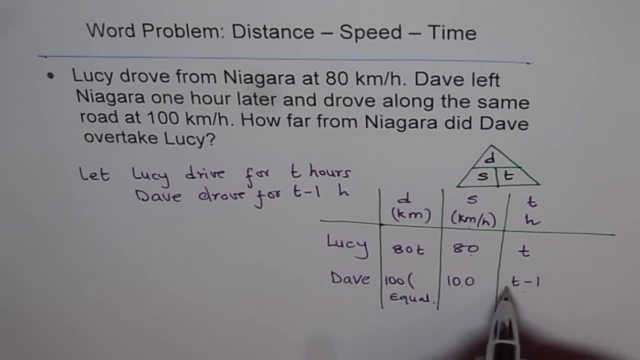 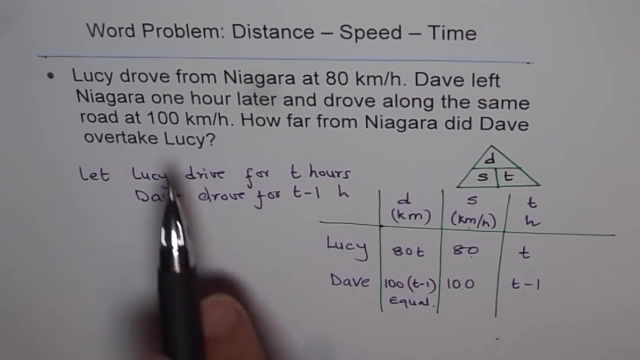 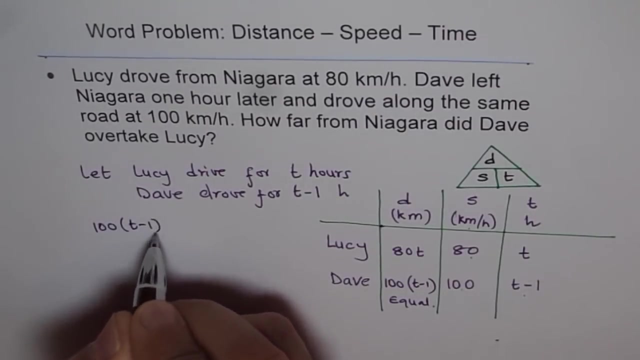 speed into time. For Dave it is 100 and time is t minus 1.. So that is how we can fill up the data from the given word problem and visualize the situation. And now we know, at the time when Dave overtakes Lucy, distance covered are same. Therefore, 100 times t minus 1 is equal to 80 t. 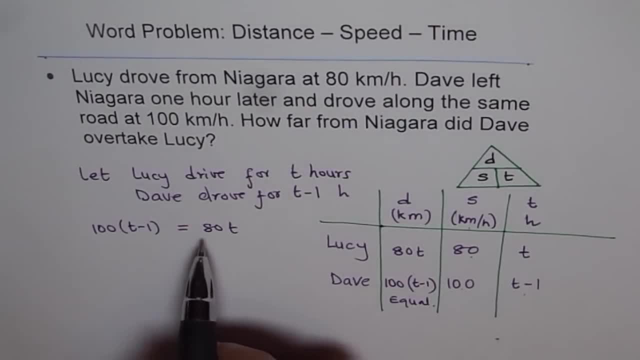 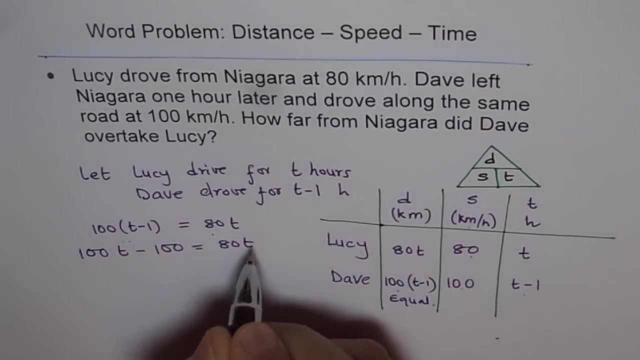 So distance covered by Lucy is equal to distance covered by Dave. So this is distance covered by Dave, right, And that is the distance covered by Lucy. They are same. Now we have one variable and one equation. It can be solved very easily, So let's open this bracket. So 100 t minus 100 equals to 80 t. Bring the. 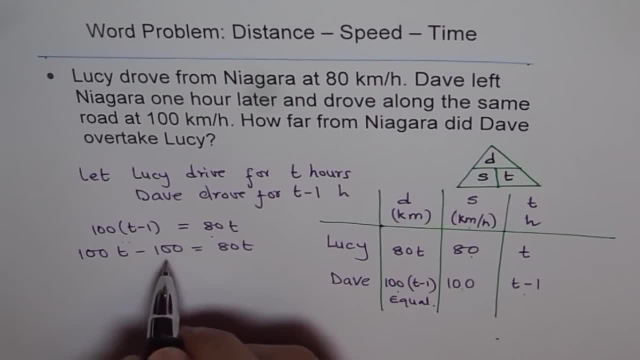 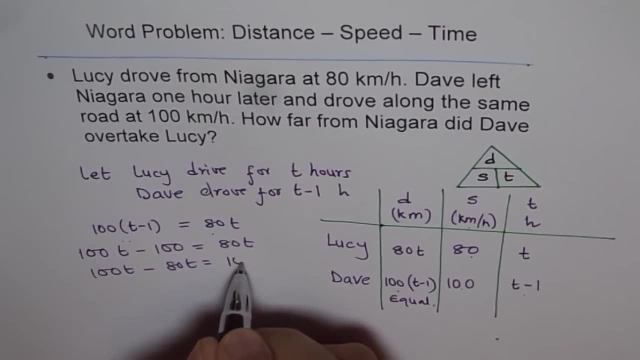 variables on the left side and constants and numbers on the other side. So we get 100 t minus 80. t equals to 100. Or 100 minus 80 is 20.. 20 t equals to 100. And t is equals to 100 divided. 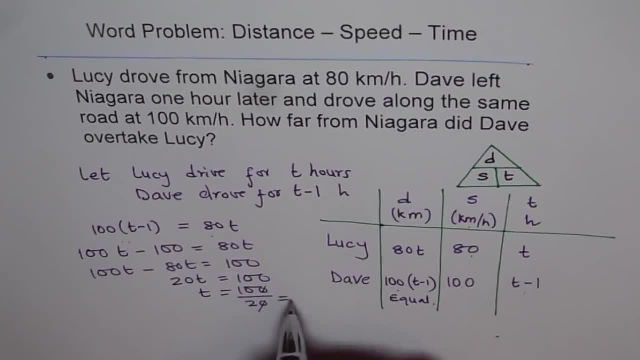 by 20.. That gives us 5.. So in 5 hours Dave is going to overtake Lucy. But the question here is: how far from Niagara did Dave overtake Lucy? We have to find distance, This distance correct. So what we will do now we know what the time is.